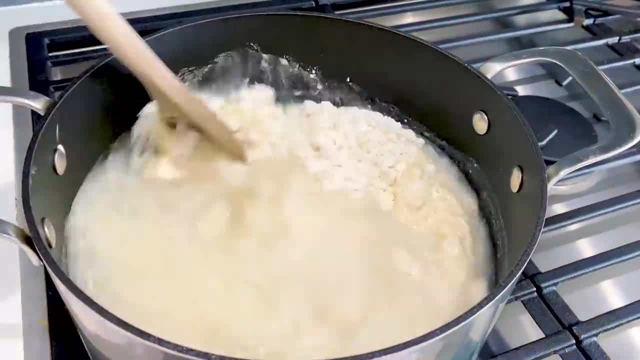 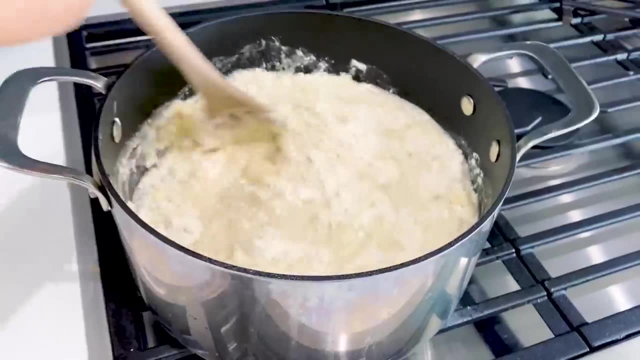 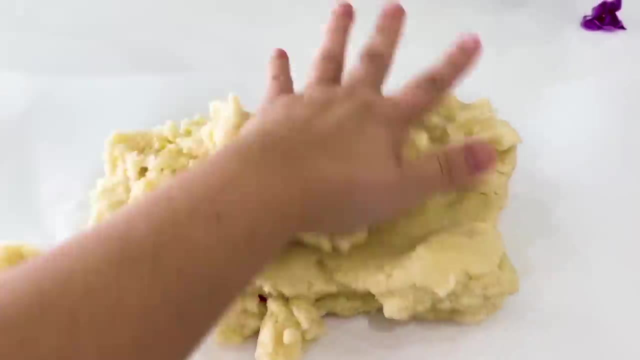 Okay, so now I'm cooking the Play-Doh on medium heat And I just keep doing this until it hardens and thickens. Whee, Okay, I think it thickens, and now I think it's ready to continue. Look, next step, after it cools down, is just to meal the dough like the bread. 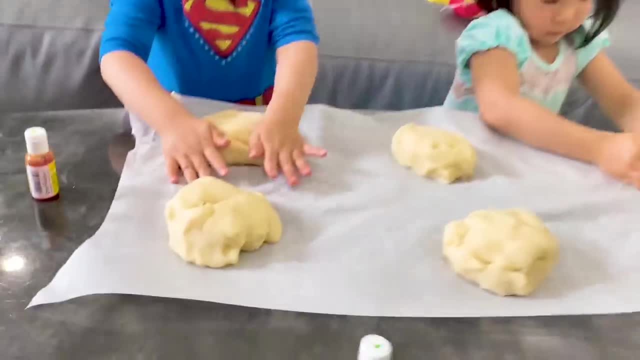 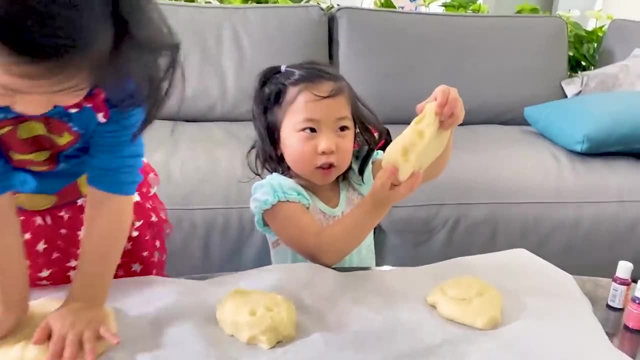 So just keep doing it until it's smooth. Woo, I got all the Play-Doh out and my cake's gonna test it. Does it feel like Play-Doh? Yeah, Mommy, it's really stretchy. Yeah, like Play-Doh. 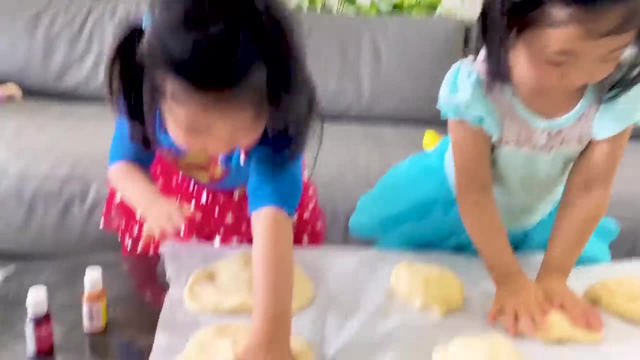 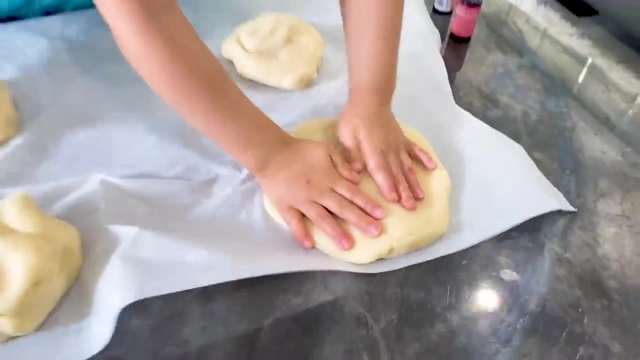 Well, it's like a pancake. Make it like a pancake. Okay, Emma wants to make each one like a pancake. Good idea, Oh, love it. I want to make mine like a pancake. Okay, You do this part. 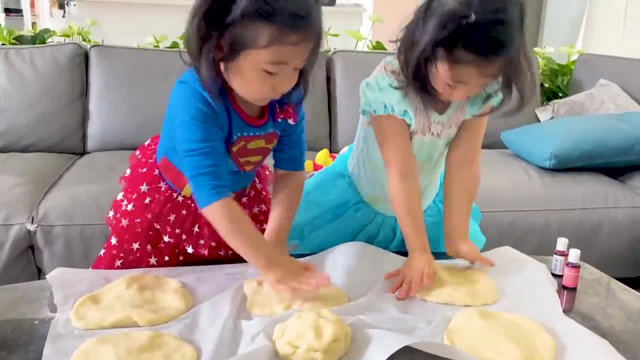 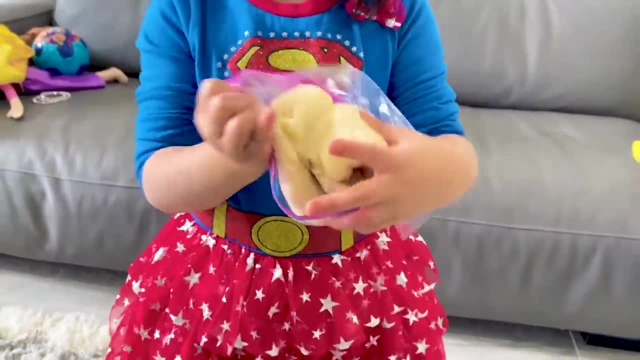 Next step is to flatten it out like a pancake. Emma says: There you go. We're gonna put each one in a Ziploc bag. Emma's helping me right now. Good job, Emma. Yeah, There you go, like that. 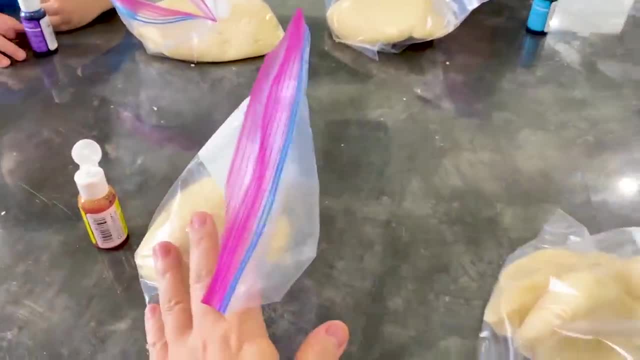 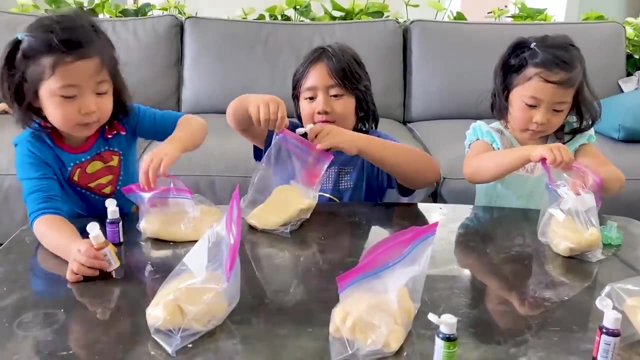 Good job. So now we put each one in a Ziploc bag, then we're gonna add color to each one. All right, so go ahead, add the colors. Can I put mine? can I put this one first? Sure, Okay. 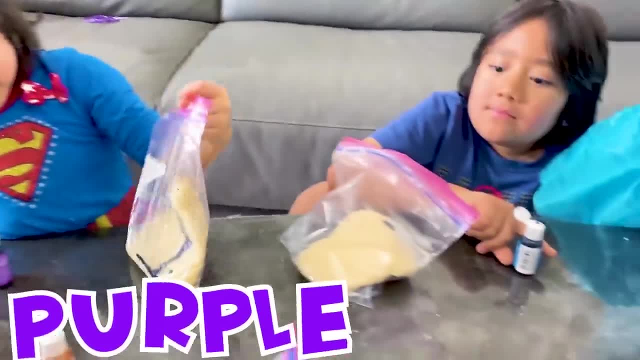 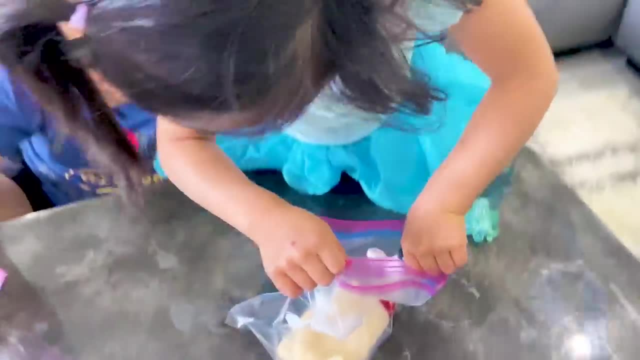 Play-Doh. Oh, there you go. So Emma put in purple, Ryan put in blue. You can add a little bit more. Ryan Purple And Kate add in pink red. There you go, Pink red, Mew it together on the outside. There you go, like Emma. 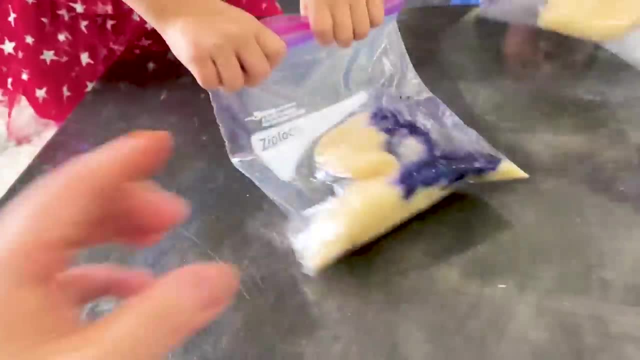 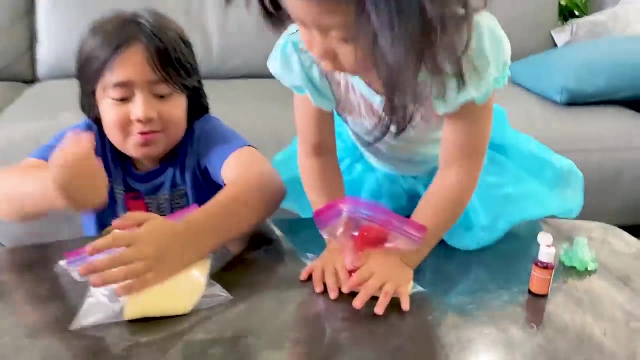 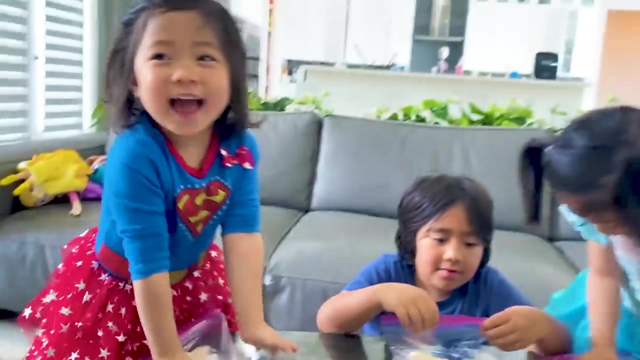 Not shake guys Like this, Like this, Just mew it like that. There you go, There you go, Good job, Kate. Yeah, There you go. Good job guys. Make a pizza. Make a pizza Feeling it like a pizza. That's right, Emma. 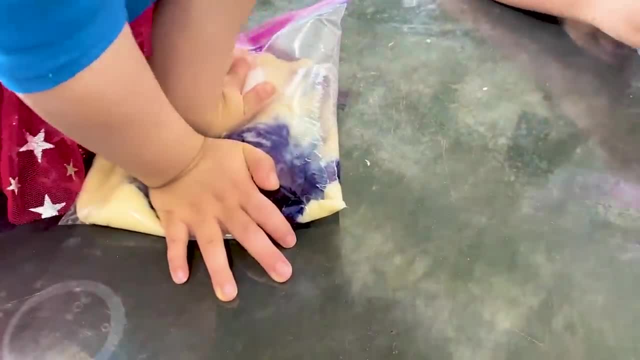 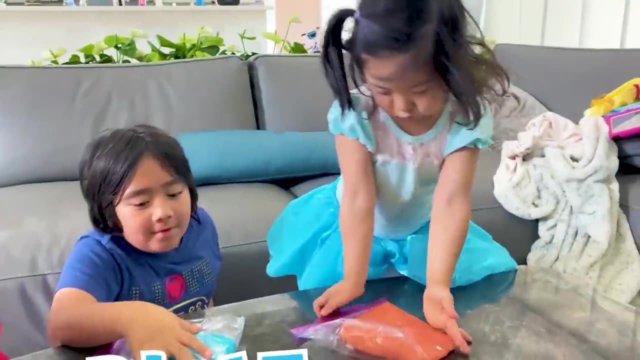 Yours is almost done, Kate. Good job Emma, you too. Good job Emma. Keep going, Guys looking good already. Look It's purple for Emma, blue for Ryan, and then I thought it was pink, but Kate was doing orange. 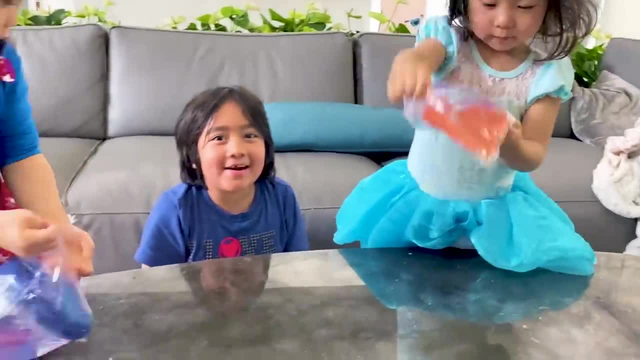 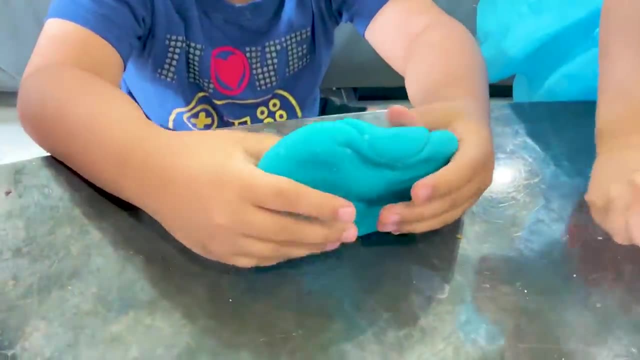 Yeah, looking good, You guys can take it out now. Actually, it feels like Play-Doh, Does it? Yeah, Homemade Play-Doh, We made it ourselves. Is this already Play-Doh, Yeah, Or is there something we need to add? 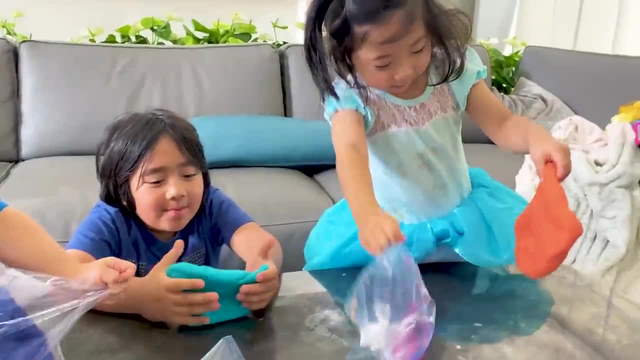 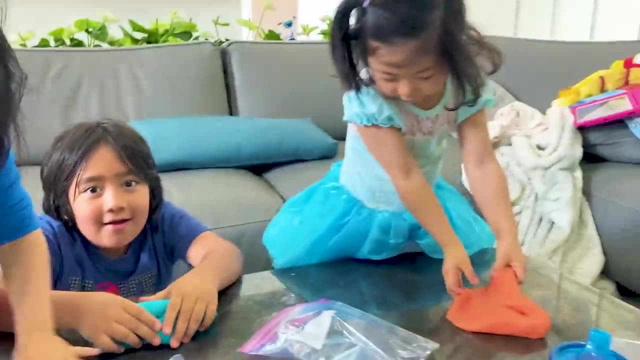 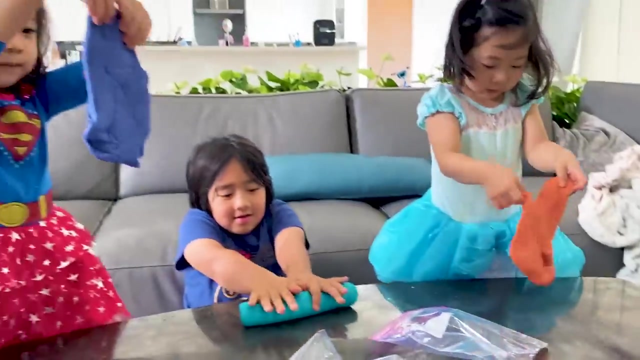 Nope, it's already Play-Doh. Wow, Play-Doh, Play-Doh. I like it, It's cool, It's cool. Yeah, Wow, I like this Play-Doh. Did you bake it? Yeah, I did, We baked it. I bake it, but you guys made it too. You guys helped me. Good job, girls. Wow, Ryan, You guys make super long. 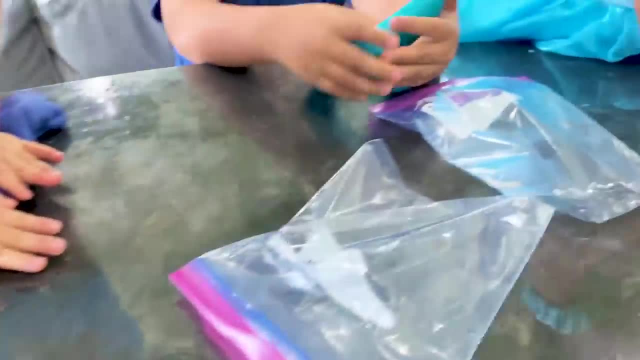 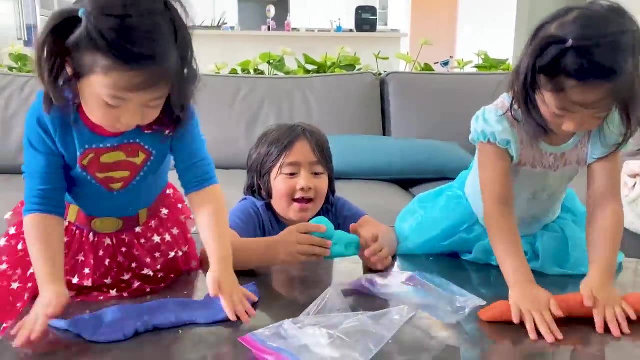 I'm making Play-Doh. I know I'm going to do whatever this is. Mom, can you buy me a roller or something? Oh, you're right, Next time I buy you a roller. Good idea, Homemade cutter, Homemade roller. 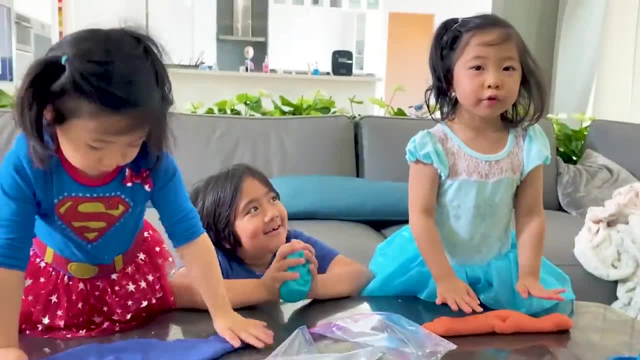 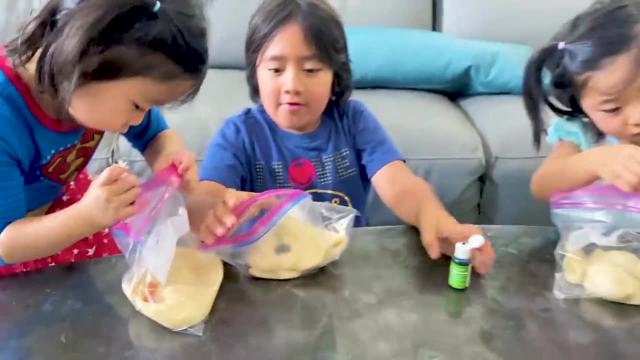 Yeah, Oh, homemade roller. What if I cut it? You're right, I need to buy rollers, Roller and cutters for next time. All right, we're going to continue making our Play-Doh: Emma's putting in yellow, Ryan's putting in green and then Kate's putting in pink. Good job, Kate. There you go. I see some color going in there, Nice. 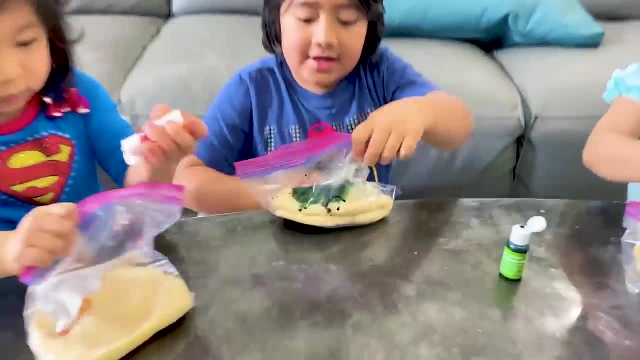 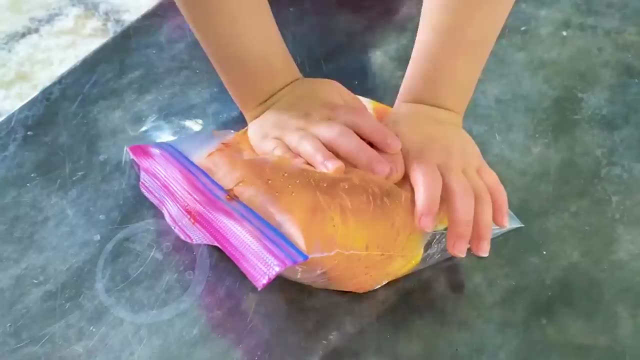 Yeah, Yeah, keep milling it. There you go. Yeah, Oh my gosh, mine went pretty far already. Yeah, There you go. Good job, Spreading it all out, guys, Spreading it all out. Good job, Emma. Emma's looking good too. All right, I'll show you guys the final result when they're done. 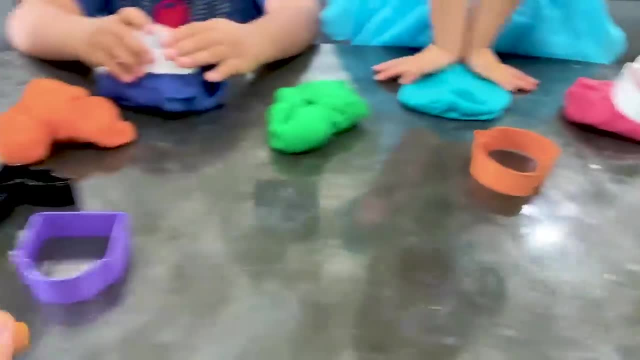 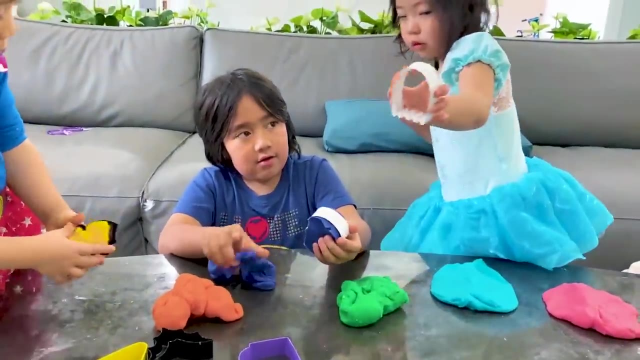 So we got all our colors already now. So we have leftover Halloween cookie cutter. We're going to use that, but you guys can use any cookie cutters if you have it. Mom, this is a ghost. Oh, that is a ghost, You're right. 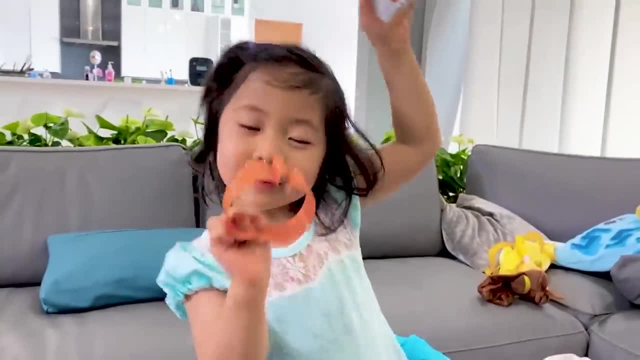 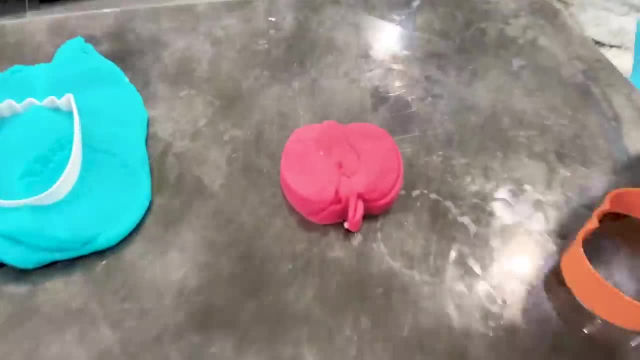 Oh yeah, that is a ghost And this is a pumpkin. That's right, Pumpkin. I see your bat, Emma. Good job, That's a bat. I made a pumpkin You did. Oh, that is a pumpkin, Good job, All right, let me see your bat, Ryan. 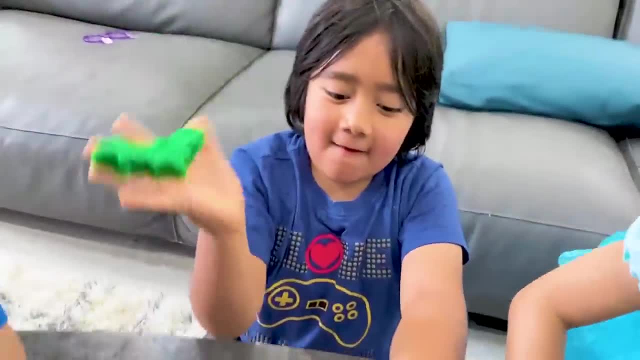 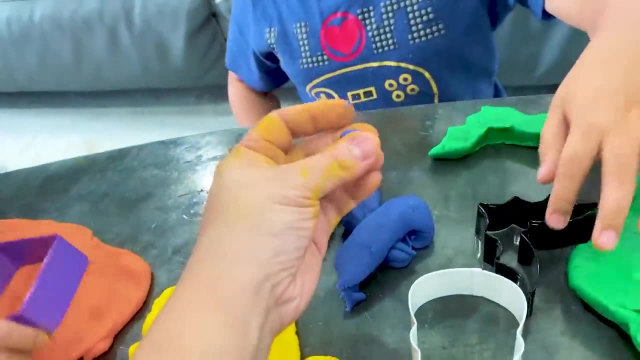 Okay, my bat is like this. Oh, it does look like a bat. Good job, All I was missing is some eyes. Good, The thing about Play-Doh is you can just get a little thing like this right and then you just make eyes. 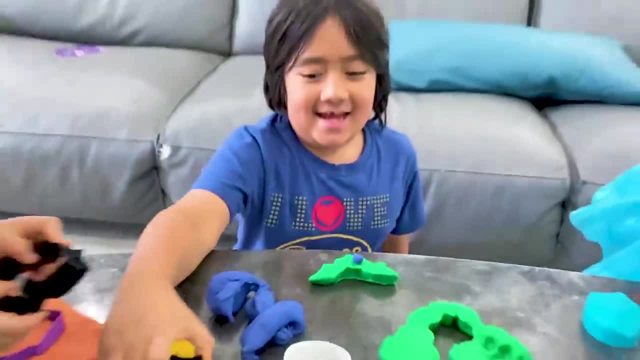 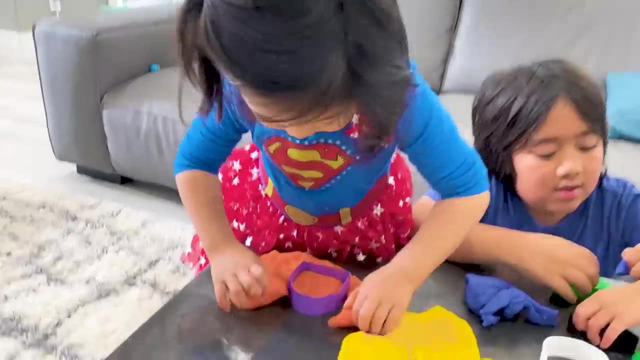 Mom, an eye. Ryan's bat has a giant one-eye bat. Can I smash it and make a bat? Sure, you can smash it. Oh, Kate smashed her bat. What are you making, Emma? I made a house. Oh, it's a house.